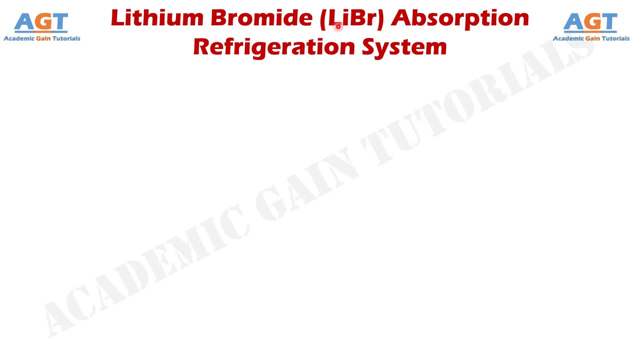 Refrigeration System, Where LIBR is the short form of Lithium Bromide. Now, whenever we talk about refrigeration process, the first thing we need is a refrigerant or coolant. We can think of a refrigerant as the messenger or traveler, Because refrigerant is the actual carrier or 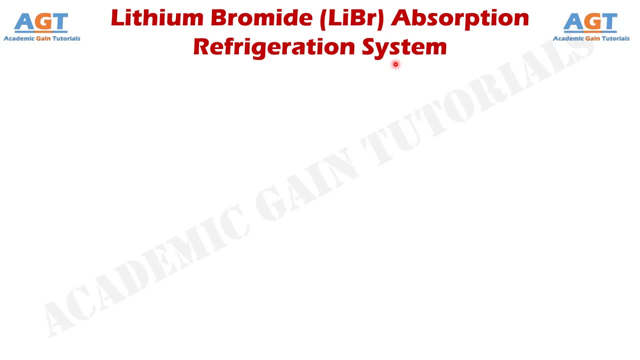 medium of heat exchange throughout the whole refrigeration cycle. Here in Lithium Bromide Absorption Refrigeration System, Lithium Bromide is used as the absorbent And we use water as a refrigerant or coolant for this Lithium Bromide Absorption Refrigeration System. So 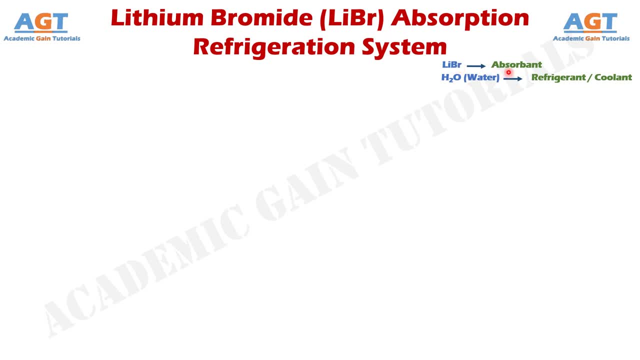 the Lithium Bromide Absorption Refrigeration System is used as the absorbent, So the Lithium Bromide works as an absorbent and its function is to absorb water, Whereas water is the refrigerant, So water gives the cooling effect. in Lithium Bromide Absorption Refrigeration System, 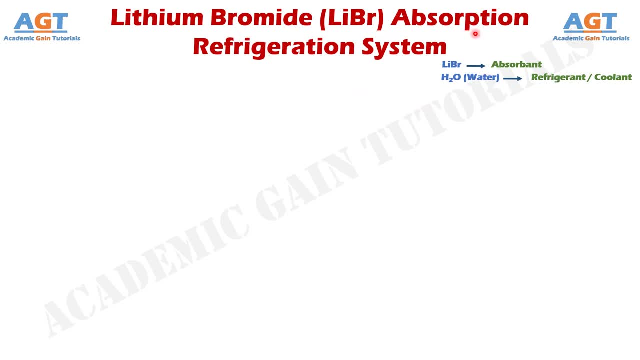 Now let's look into the major parts and components and basic working procedure of Lithium Bromide Absorption Refrigeration System. First of all, here we have an absorber. Inside this absorber we have a solution of Lithium Bromide and water. 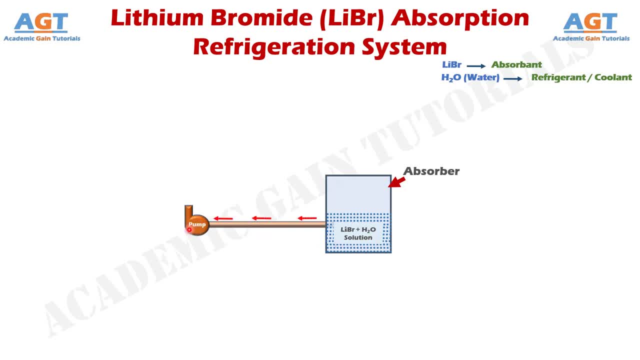 Now, beside this absorber, there is a pump. Using this pump, we will pump this solution of Lithium Bromide and water from this absorber to this generator. So the function of this pump is to transfer the solution from the absorber to the generator. Now, when the solution of Lithium 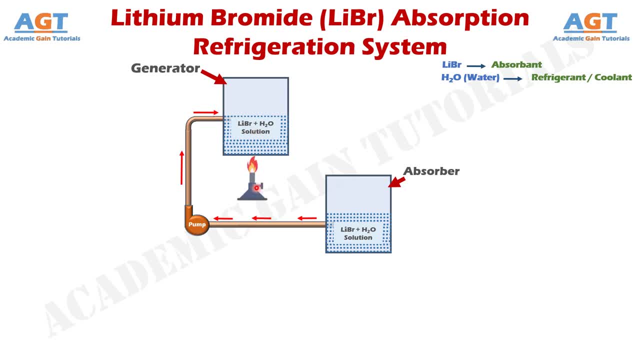 Bromide and water reaches the generator. here we have a gas burner And using this gas burner we provide flame and heat to this solution of Lithium Bromide and water. So the function of this gas burner is to provide heat to the generator And when heat is applied, to this solution, 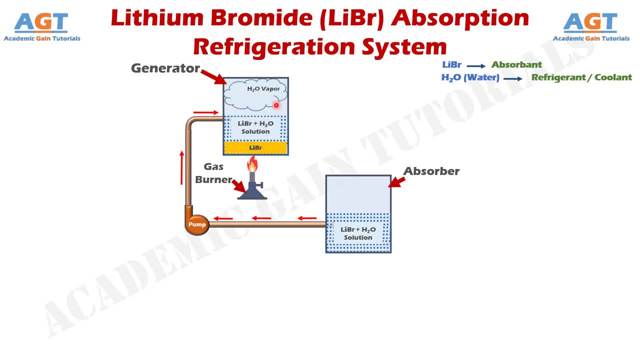 water is converted to vapor, And when water from this solution turns into vapor, only Lithium Bromide is now left in the generator and accumulated here. Then the generator sends this Lithium Bromide back to the absorber through this connecting pipe. After that connected to the generator, we have a condenser Now from the generator. this: 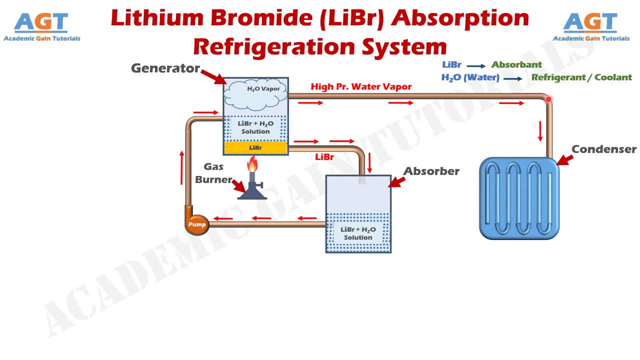 high pressure water vapor will be passed forward and sent to the condenser through this connecting pipe. When high temperature, high pressure water vapor enters this cold condenser, then the condenser absorbs the heat from the water vapor and converts it into liquid. In practical use, the condenser 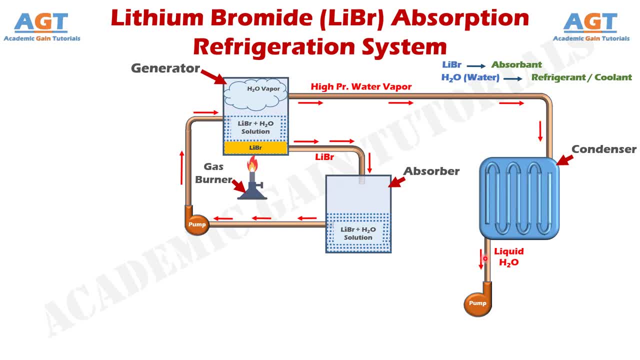 cannot convert 100% of this vapor into liquid And there will be a mixture of liquid with partial vapor. Most of it will be liquid and some of it will be partial vapor. But the prime purpose of condenser is to condense this water vapor from vapor to liquid. This condenser can be water cooled or cooled by any. 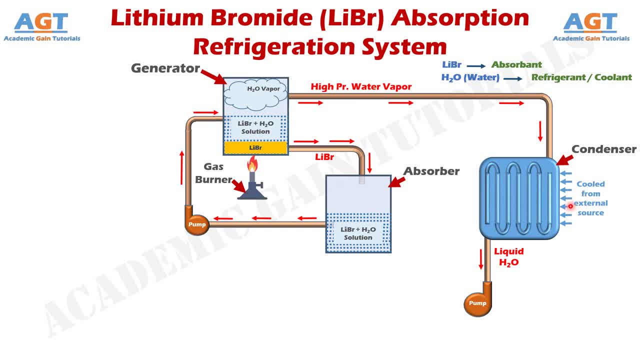 other substance from an external source which will liberate the latent heat of this vapor coming into the condenser and thus condensing keeps happening. After that, these condensed liquid will enter this pump. The pump will send this liquid through this throttling valve. We can also call it an expansion valve. Now, this high pressure liquid coming from, 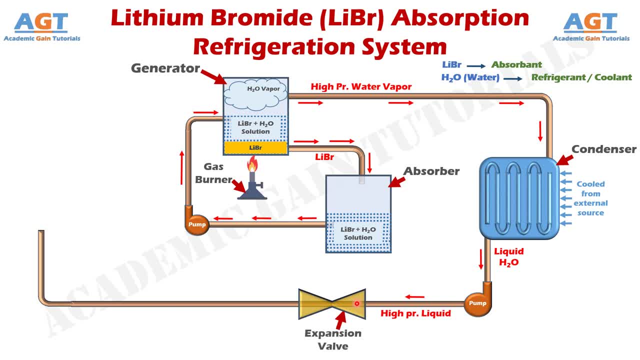 the pump will be expanded inside this expansion valve. We know that when expansion occurs, the pressure between the molecules decrease considerably. thus the temperature falls. So this high pressure liquid will be expanded into low pressure, low temperature liquid. Thus here we get very cold, chilled, low temperature liquid coming out of the expansion valve. Then this liquid will be 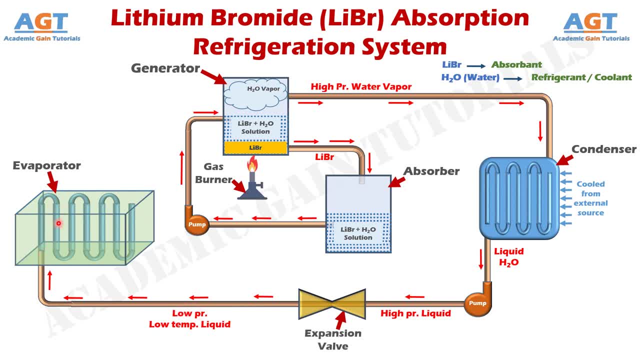 passed over to the evaporator. We all know that the main cooling effect or refrigeration effect will be in the evaporator. We all know that the main cooling effect or refrigeration effect will be in the evaporator. 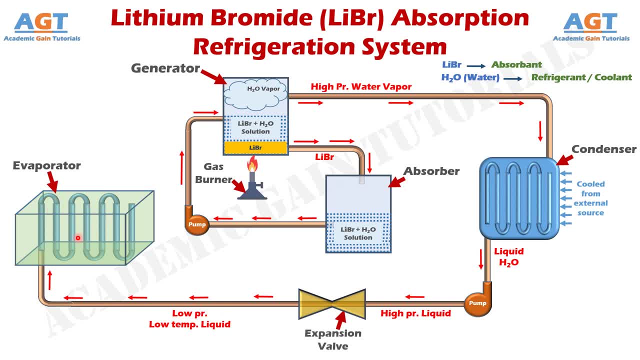 So when this low pressure, very cold, chilled, low temperature liquid will enter the evaporator coils, it will absorb all the heat present in the surface of the evaporatorudge By absorbing all the heat from the surrounding surface of the evaporator coils, this cold 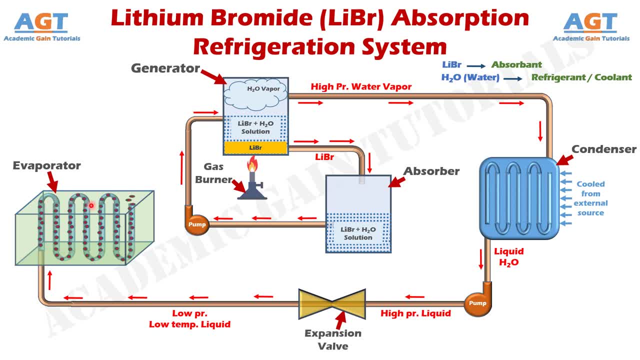 chilled water will turn into low pressure vapor inside these coils and the surrounding surface of the evaporator will become cold by losing the heat to this liquid. Thus the cooling effect, or refrigeration effect, will be on the evaporator. This cooling effect, or 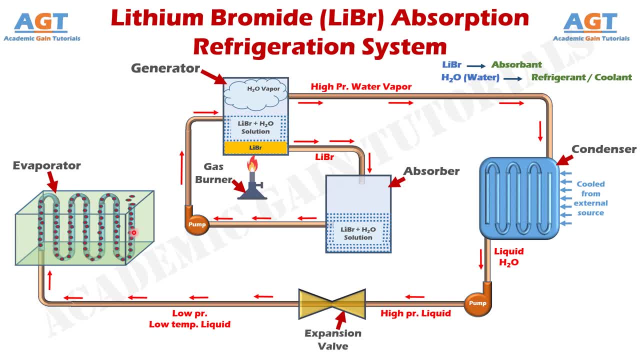 effect has occurred. after that this low pressure water vapor will leave the evaporator and enter the absorber again through this connecting pipe. then again, this low pressure water vapor will form a solution with the lithium bromide present in the absorber. the pump will again send this solution to the 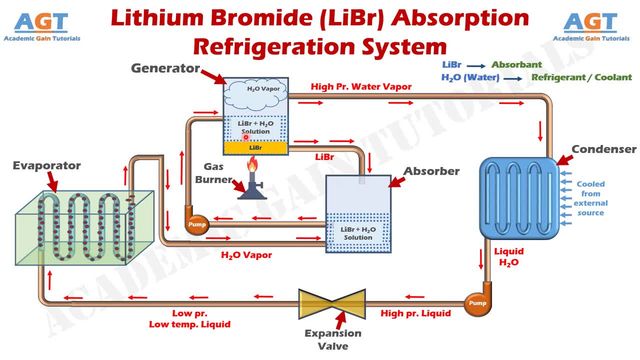 generator, where the water and lithium bromide will be separated again by heat and the whole process or whole cycle will keep repeating again and again. thus, refrigeration will be happening continuously in the evaporator. so this is how a lithium bromide absorption refrigeration system works. thank you for.